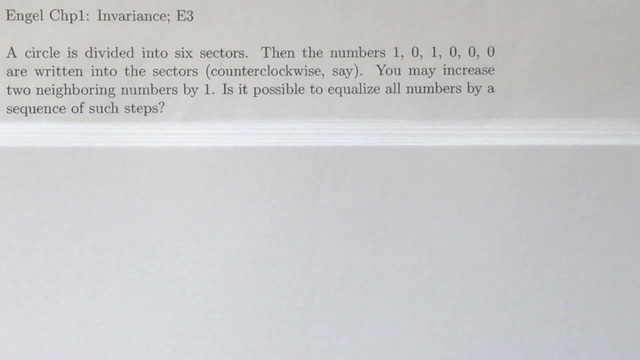 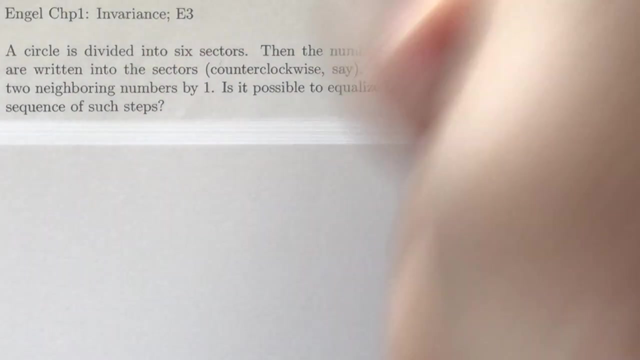 Hello, fellow problem solvers. So today we're going to be doing a problem from the Engels book on problem solving strategies, chapter one, invariance, example number three. I suggest you try this problem out for a minimum of 10 minutes, ideally 30 minutes, but not more than an hour. If, on the other hand, you'd like to go along with us, I suggest you read the problem, put your first ideas out on paper for the next five minutes, And now let's begin. So before we begin the problem, I want to point out what this principle or invariance, 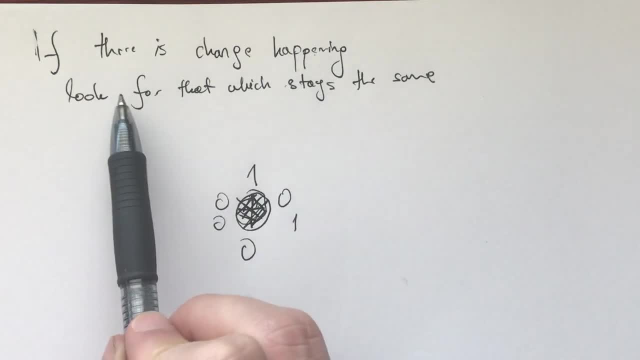 is. That is saying that if there's a change happening, look for that which stays the same. And here in this problem, we are allowed to increase the size of two neighboring numbers by one. So when we are doing that, when we're say increasing like, say, these two neighbors to one, 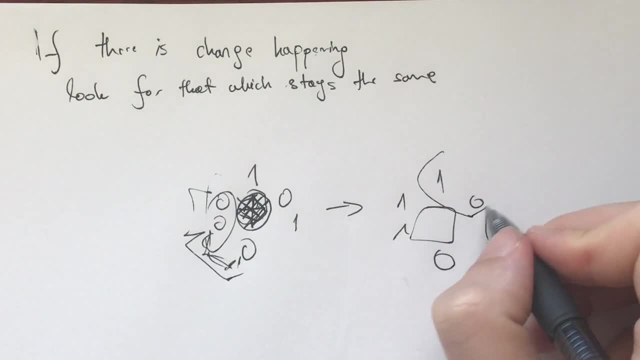 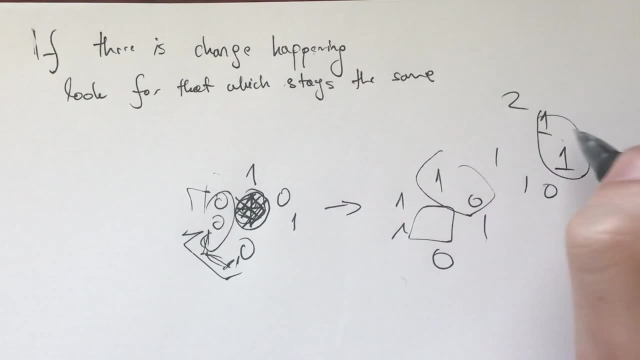 now we have one, one zero, one zero, And then we say: increase these two neighbors, we'll get two: one one zero, one one. Then we say: increase these two neighbors, and then we get all. 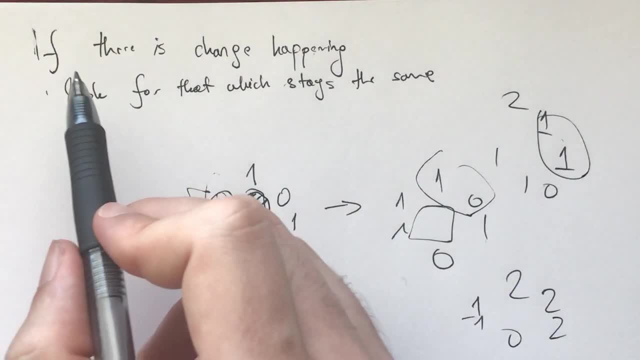 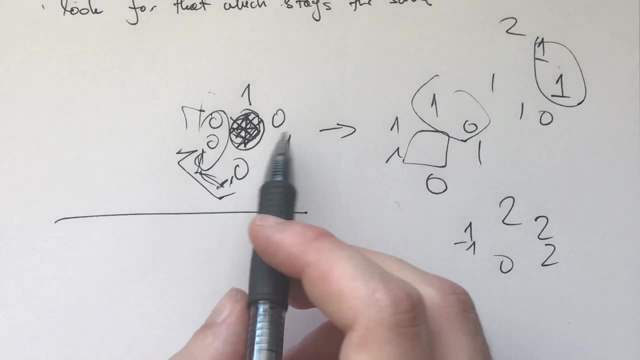 two, two, two, zero, one, zero, And then we say, increase these two neighbors and then we get all one. can we at some point get to a place where they're- all of these numbers are equal, and the thing to look for initially for you is, as we're increasing these neighbors by one, what remains? 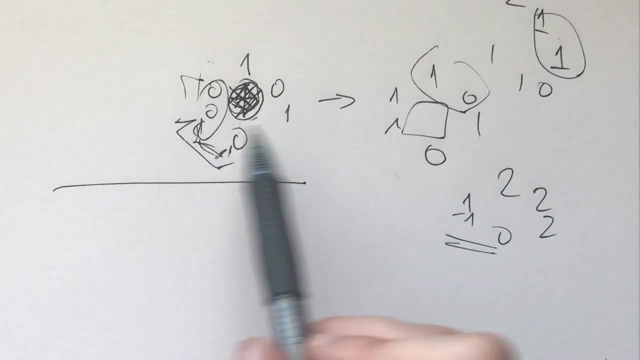 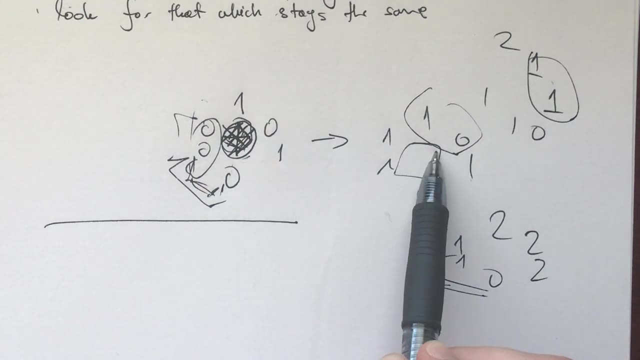 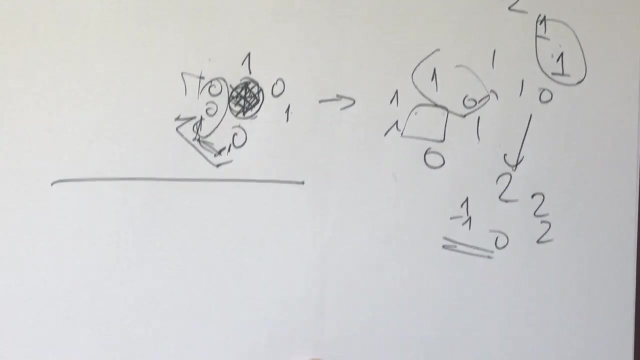 the same, and i invite you to take five to ten minutes and figure out what remains the same here, throughout all of these different cases. so what is the same with here and here, and what is also the same here and here, here and here. what do all of these things have in common? if anything, i invite 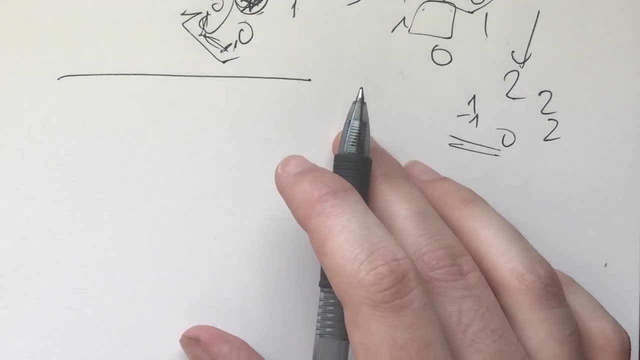 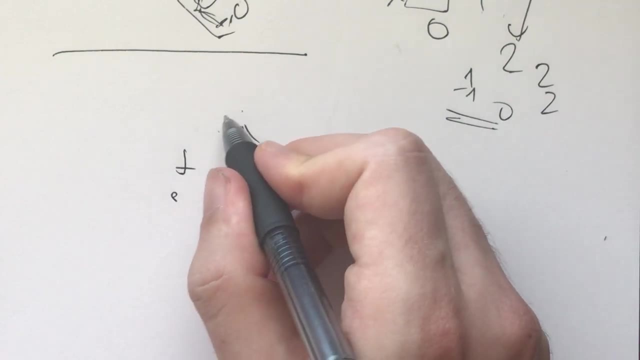 you to take those five, ten minutes and figure that out, and the way to look at this in general is to look: okay, you have these numbers- a, b, c, d, e, f- and what you may do at any point is you may increase a and f, so then both of these will be increased by one or f and e, e and d, d and c, b and c, or a and b. 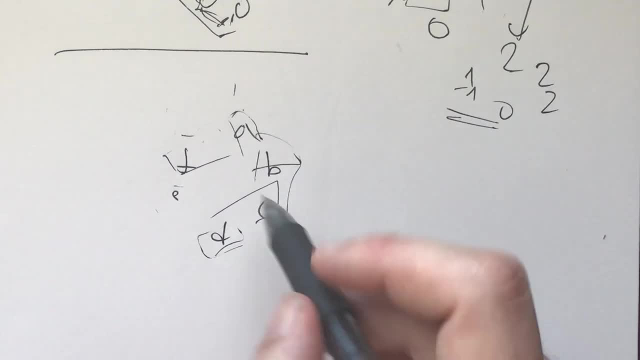 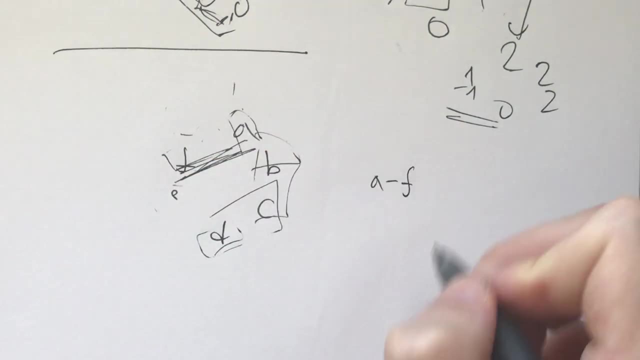 now, in each of these instances, what is something that's not changing? well, if you increase a and f, then the difference between a and f remains the same. if you increase f and e, the difference between e and f remains the same. e and d if you increase them. 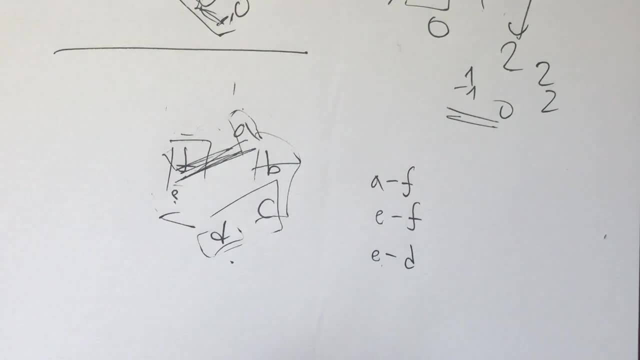 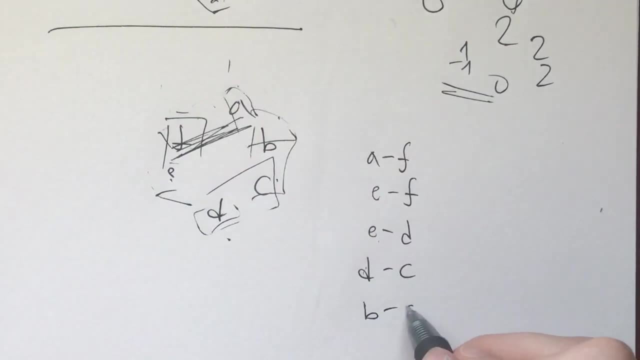 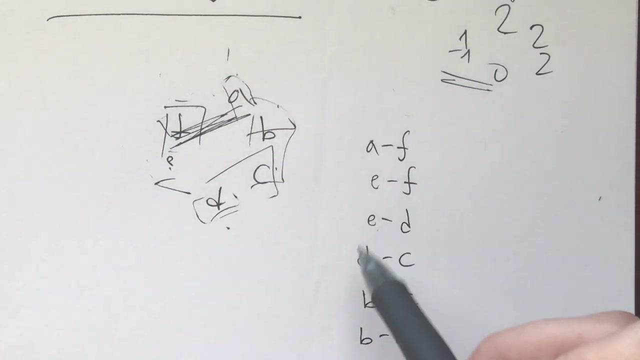 the difference between e and d remains the same. if you increase d and c, the difference between them remains the same. b and c: the difference between them remains the same. b and a: the difference between them remains the same. so now, what remains the same, regardless of which one of these we 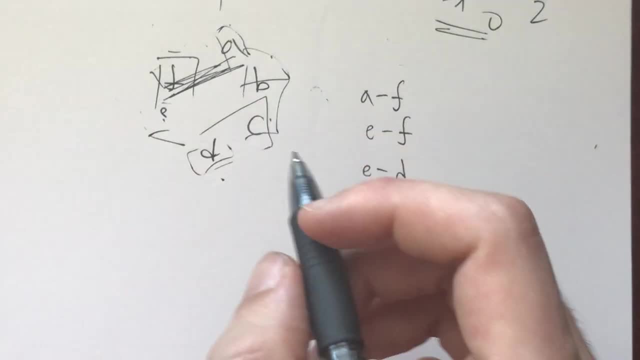 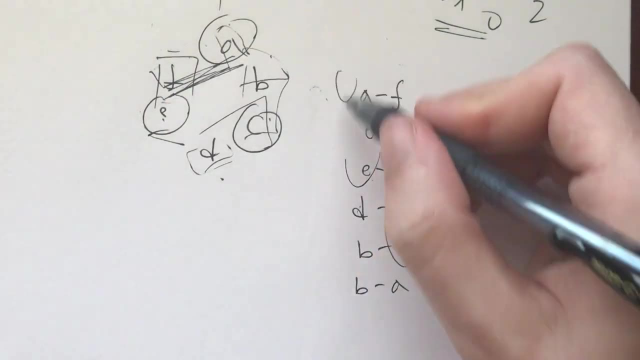 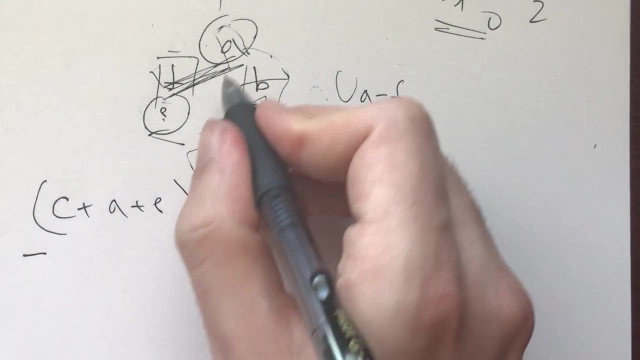 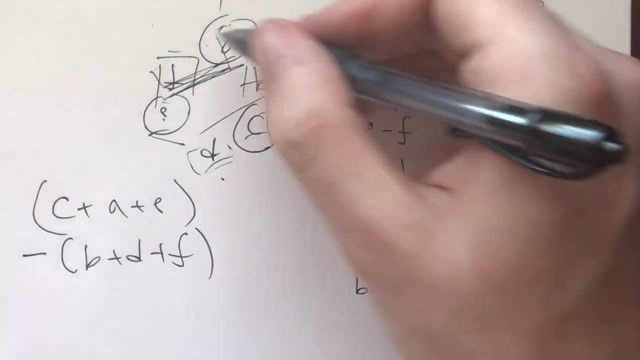 increase. i invite you to take three minutes and think about that. and the answer is the difference between c plus e plus a. so once you take all of these on one side, so c plus a plus e, the difference between this and b plus d plus f always remains the same, because that is what we can capture in. 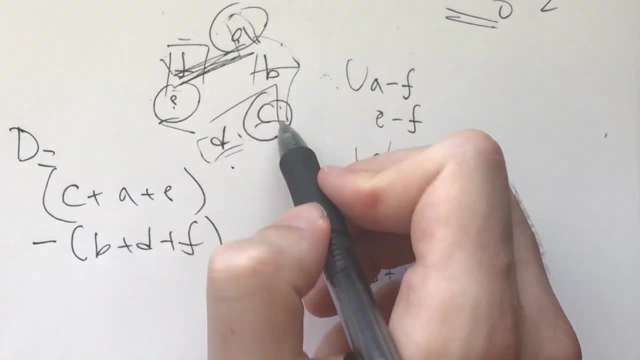 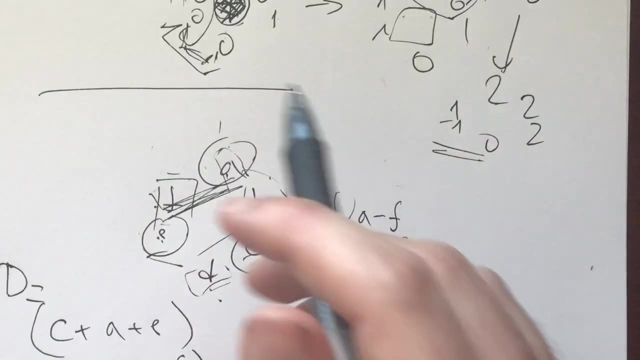 this sort of difference. here, the difference between a plus c plus e minus b, minus d minus f is always the same. and now, looking at our problem, what would it mean for all those numbers to be equal? well, it would mean that this difference here is equal to zero. but what is the difference? 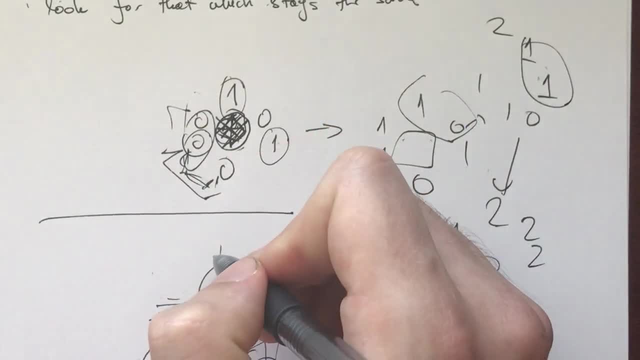 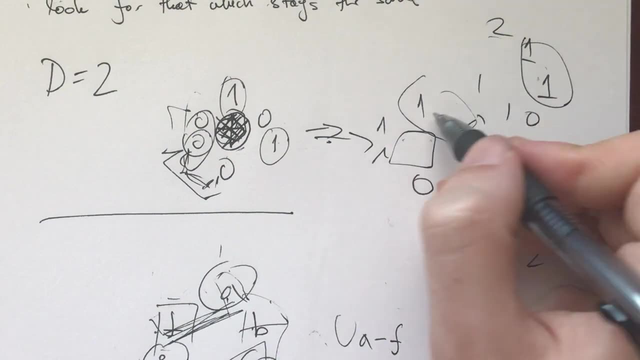 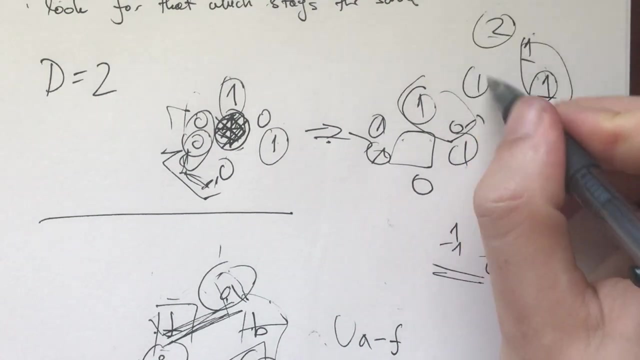 initially. well, the difference is one plus one plus zero minus zero, minus zero minus zero. the difference is initially two. that means it will stay two, like when we go here again look at it, it's one plus one plus one minus one, which is two. now look at here: it's two plus one plus one minus one minus one. it's two. and here again it's two. 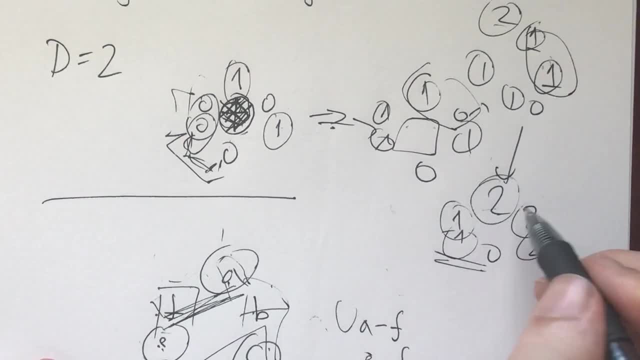 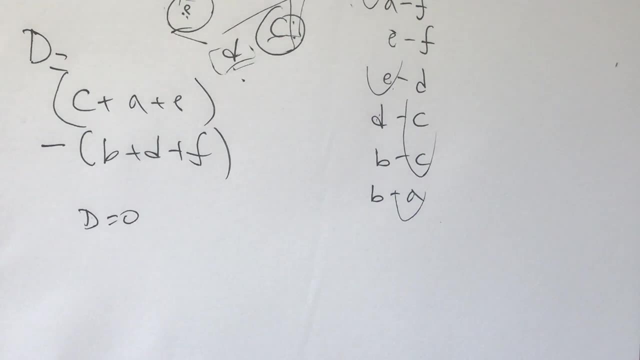 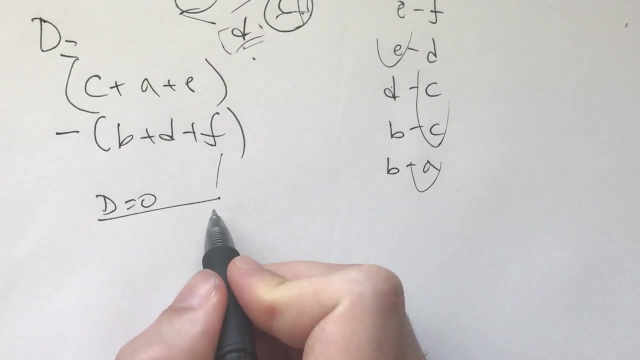 plus two plus one minus one minus two, it's two again, so it always remains two, and this means that we can't ever get to a place where all of these numbers are equal. this is the first video in our principles of invariance, and i never, like you, can try to write a solution yourself. it shouldn't be that, that you just need. 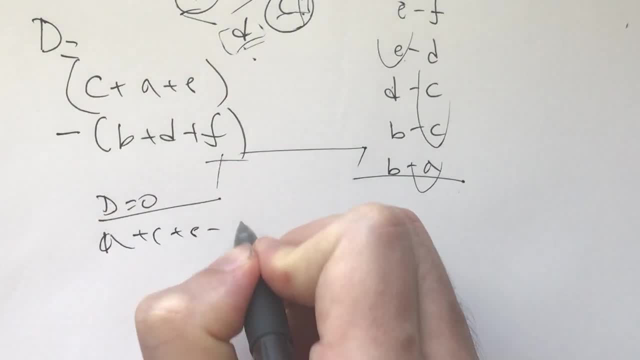 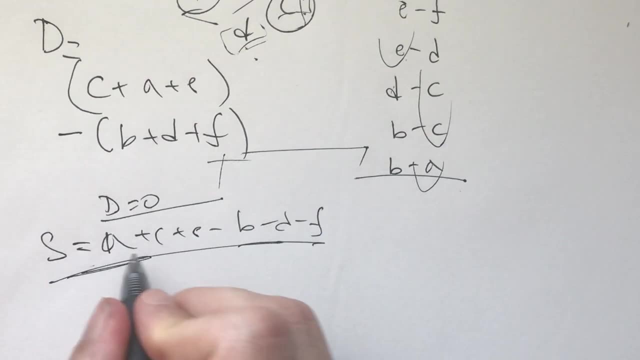 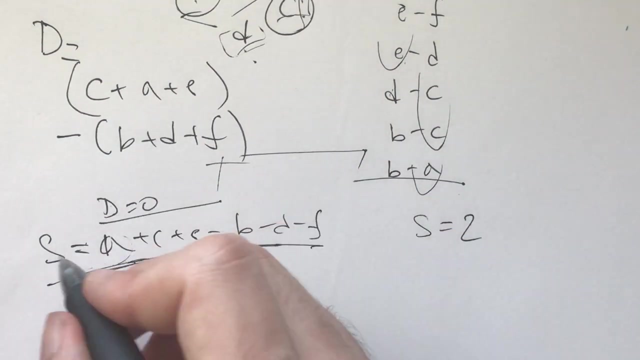 to call this thing: a plus c, plus e, minus b, minus d, minus f. you just name this, sum s and you say: notice that no matter which you neighboring numbers we change, s remains the same. initially, s is equal to two. if we were ever to get all these numbers equal, s would be zero. we can never.